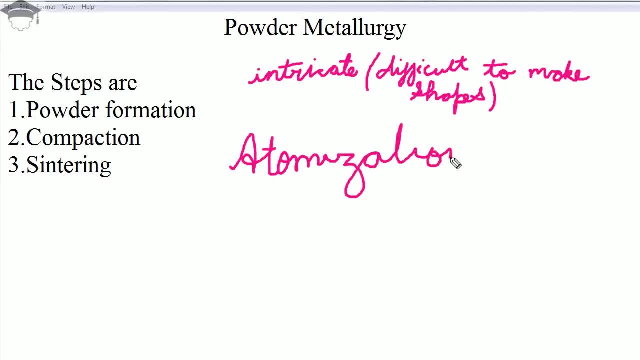 Now atomization. as the name suggests, that means we have to break the metal into very small parts, near about atomic scale, By using some techniques. what happens? we first melt the metal, the powder for which we want the metal powder that we want to form. we take the molten metal of that material, that metal. 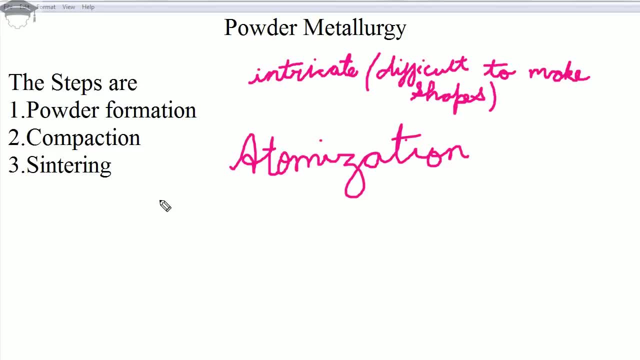 and then we spray- This is the molten metal, suppose- and we make it to fall from some height. This is the molten metal. Ok, This is the molten metal complete, and this is made to fall from a height and we have some sprayers, very fast blower or sprayer, you can say. that pushes, that sprayers are. 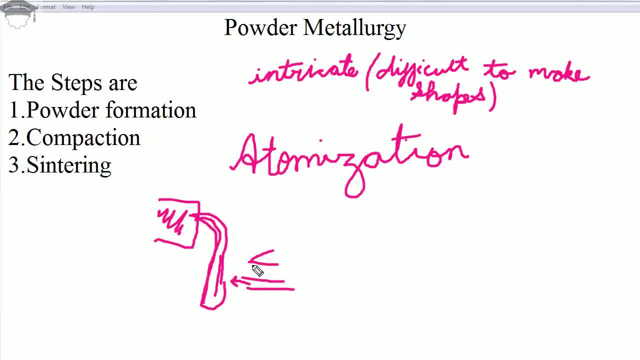 very strong jet of wind. Now, when wind is projected here, then what happens? very small particles, they are blown by the air and we have this plate here, very cool plate, and when the particles they are traveled like this and they condense on the plate and they cool down. 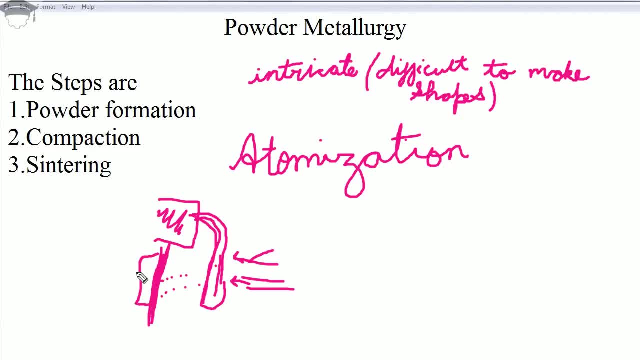 And we have a vibrator attached here which periodically vibrates this plate and the molten material. that is the molten metal. it atomizes by using the air. this is the air, this was the molten metal. it is made to fall from a height. Here it is supplied through a nozzle or blower and it pushes some amount of the molten metal. 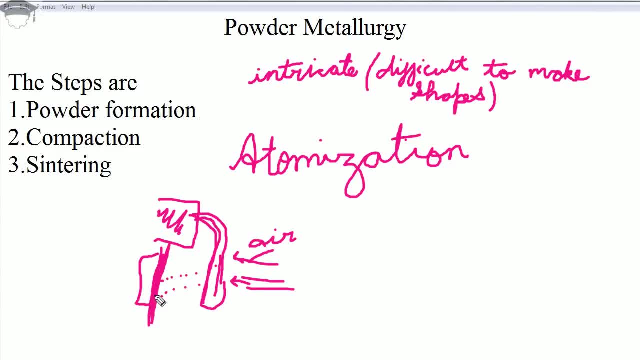 very small particles. and this is the condensing plate or cooling plate on which the molten metal, in the form of very small powder form, it drops, it condenses and this is the vibrator with it, which is attached to a vibrating motor. So the periodic this is collected in a pan. 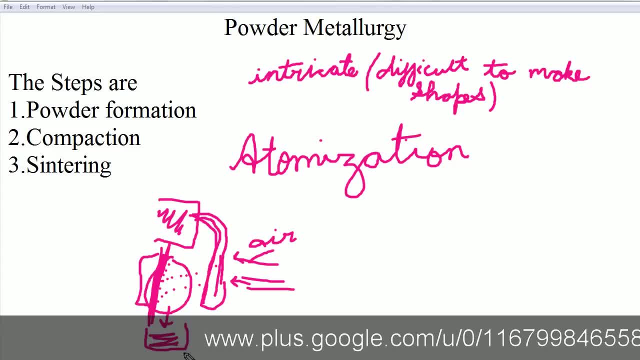 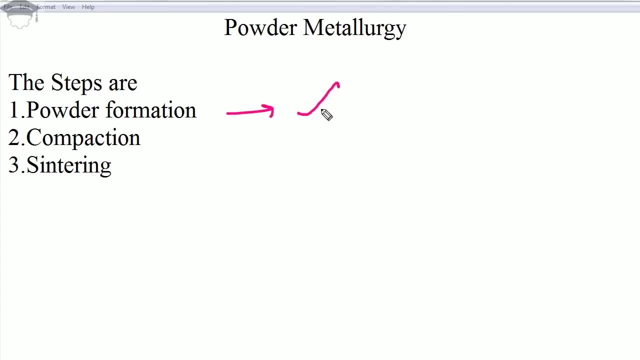 So the powder is formed. I hope I have explained atomization process. this is the powder formation. Other method can be of powder formation can be using centrifugal method. that means using the centrifugal force, centrifugal force or centrifugal method of atomization in which 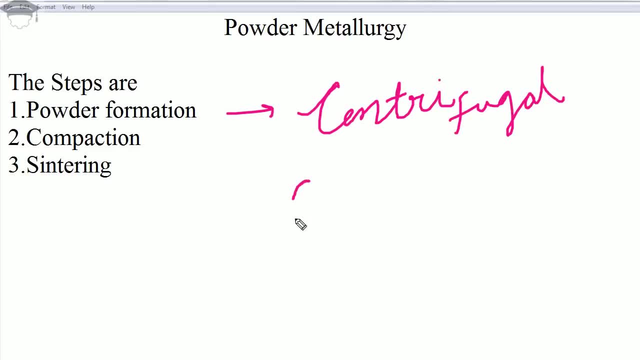 what happens? We have a molten metal In a bowl, you can say, and this bowl, it is attached to a motor spindle and this rotates at very high speed. So what happens? that the molten metal, in the form of very small droplets, it travels along. 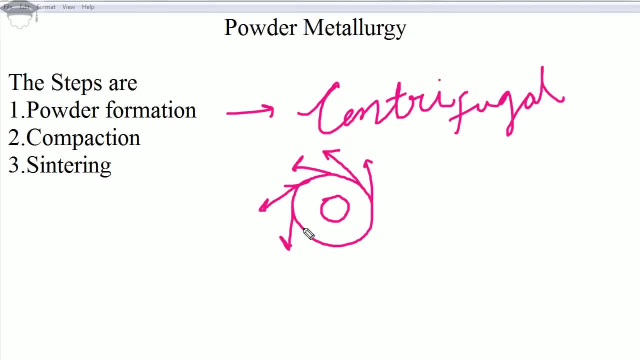 the periphery and it detaches from the molten metal and in the contact of the air, when it gets contact of the cooling air. So what happens? It gets separated and we have a large basin attached. it condenses here. All right, powder is generated, the centrifugal force, it has the particles to condense and 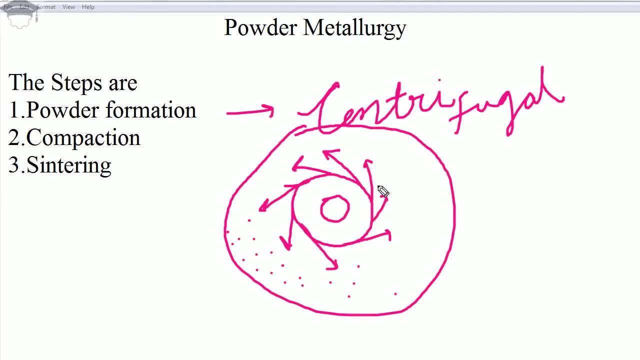 it throw off along the circumference of the bowl and these particles they condense on the secondary bowl, outer bowl, And They can be tapped and they can be collected in a pan later. So this is the first step, that is the powder formation. Second is the compaction. 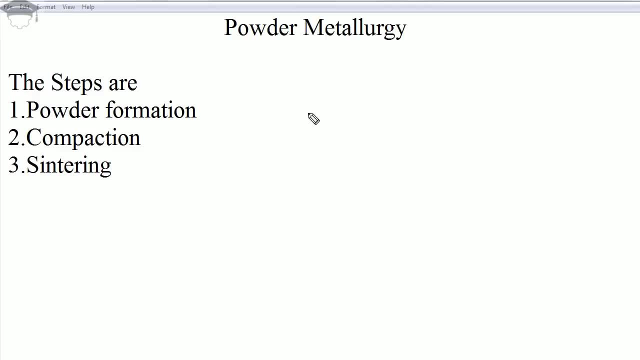 Now, any component that we need to make. we first make a die. suppose this is a die that is required, and the final shape we are going to obtain will be this, This shape We will be going to obtain. Okay, This is the component shape. all right, this blue dotted line, this is the component shape. 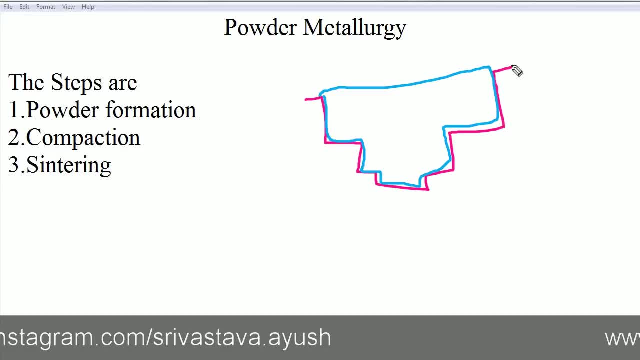 and the red. this is the die. So what happens in the compaction? we put the powder, We put the powder in the die, like this was the die. So we put the powder And It is completely filled up to the top surface. the powder, it is completely filled and the 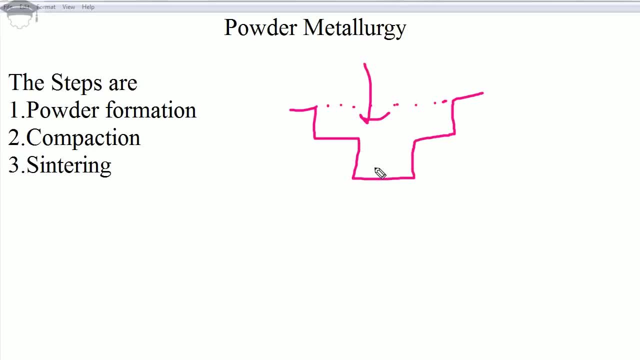 die, it is slightly vibrated so that the air between the powder that escapes and the complete filling of the mold or cavity, or you can say the complete die, is filled with the powder. Then what happens? that we supply very large amount of heat And 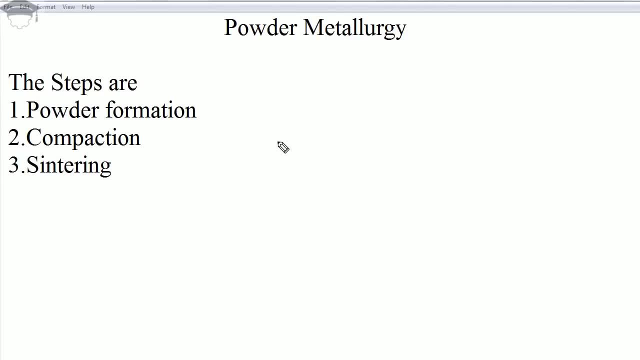 We Add very high temperature To the die. This die when it is completely filled with the molten powder. then we supply a very huge amount of heat through a burner or a furnace, and temperature above, above around 500 degrees Celsius. it is maintained for about 10 to 15 minutes. 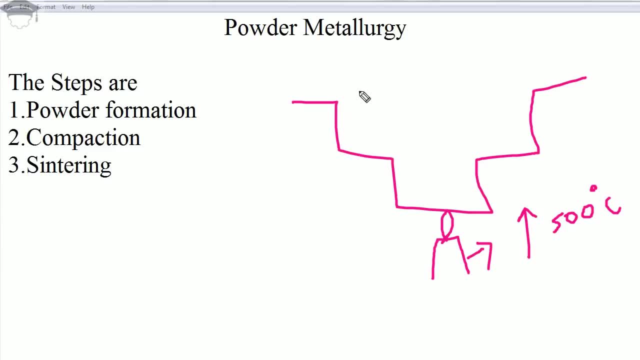 Then what happens? The metal powder, it again melts, and the metal atoms, they form the bond, bonding occurs, and so the metal powder, it forms a solid shape And finally we get the required component, like this, And the temperature and the time for which the flame is applied, it depends on the metal. 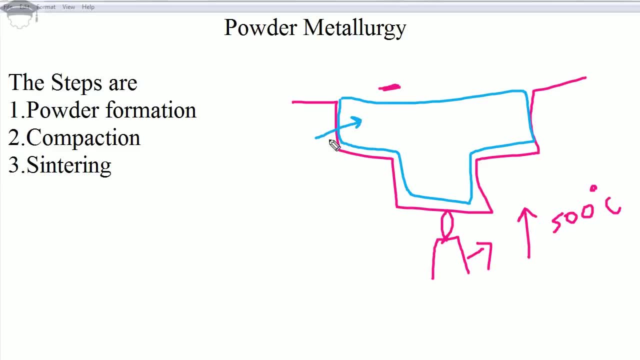 that we are going to The main metal. whether for aluminium the temperature is lower, for tungsten, temperature is higher for gold, or so for different materials, the temperature and the time for which the flame is applied in sintering process, it can vary, but the general procedure, the general process. 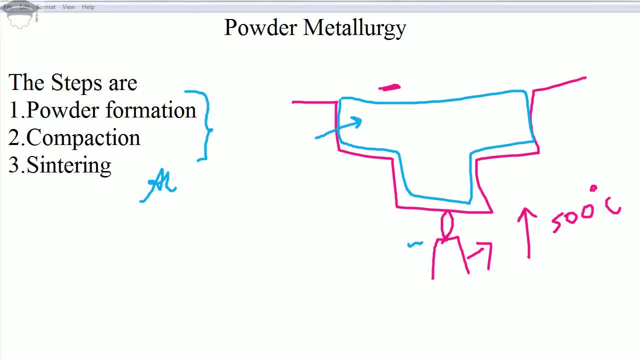 and the steps. they are these three And I hope you have found the video helpful. if you have found the video helpful, please press the like button. please share my video on social media and please check the description once for more of my social media links and other video links. do follow on Facebook, Google plus. 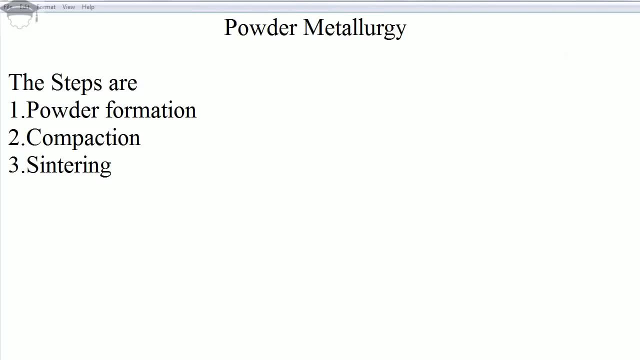 Twitter, etc. all the links are given in the description. please check the description once and if you have already not subscribed, please subscribe my channel and you can watch other videos appearing on your screen right now also. I will be seeing you in the next video. till then, take care, bye, bye. . . . .